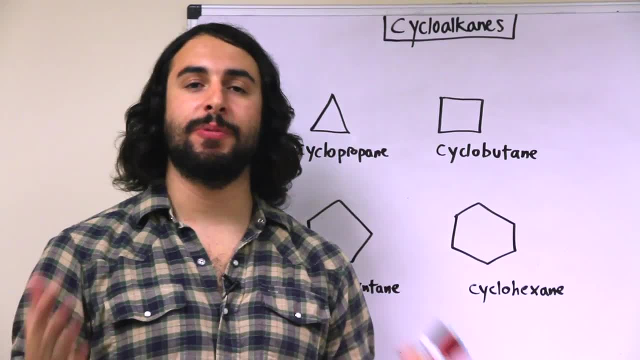 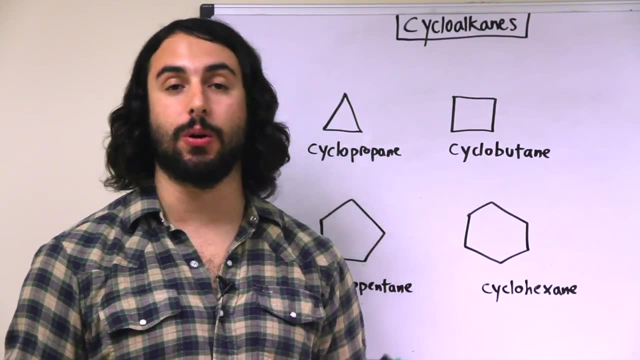 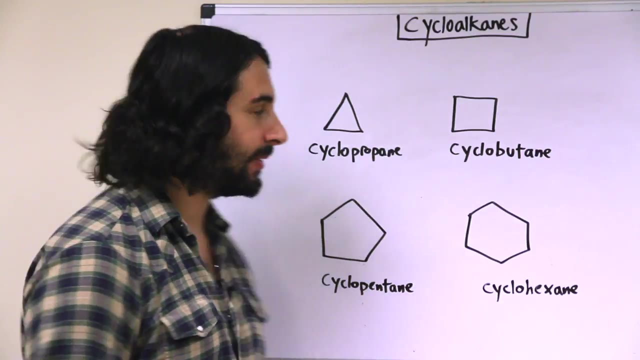 so up until this point we've been looking exclusively at linear compounds. but molecules can also form cyclic structures that we call rings. so here we can see some kinds of cycloalkanes which end up just looking like these fun shapes. so basically all the rules are the same, but for a cyclic compound we 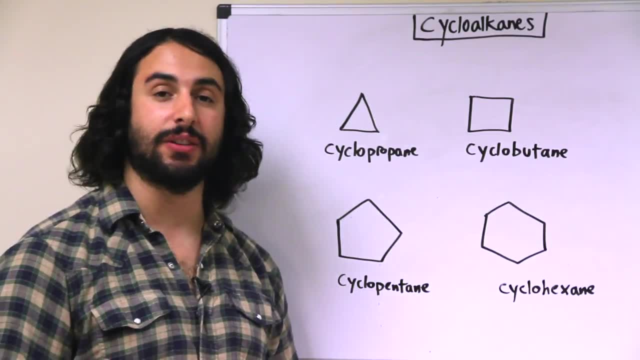 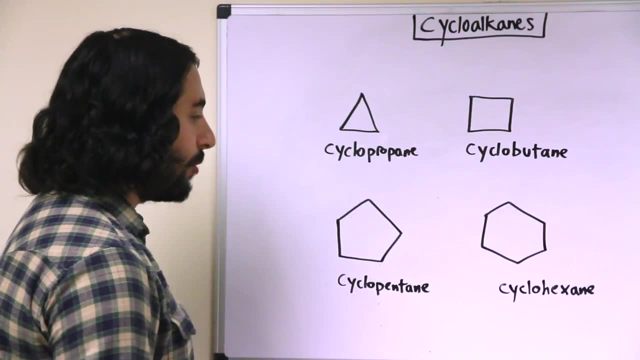 are going to utilize the prefix cyclo to indicate that it is cyclic, but the rest is the same. so a three carbon ring is a cyclopropane. for cyclobutane, cyclopentane, cyclohexane, etc. we would use the same prefixes indicating the 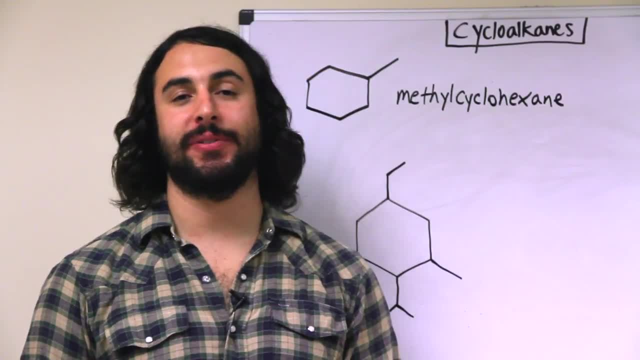 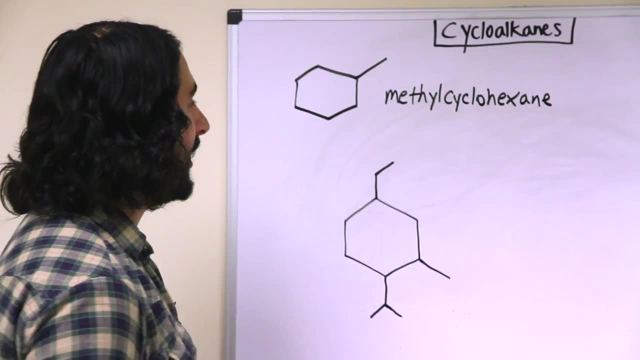 number of carbons that we already know. now let's see what happens when we're looking at cyclic compounds with substituents. so let's take a look at a simple example. here we have a cyclohexane with a methyl substituent. now 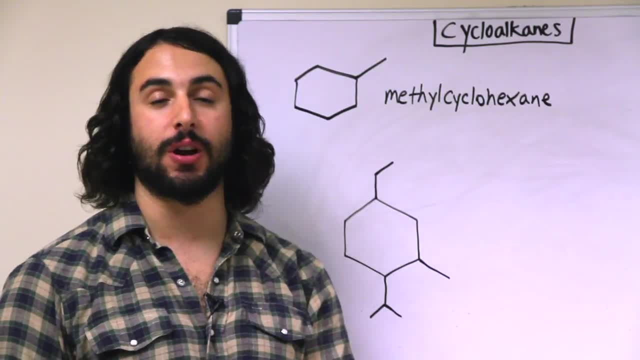 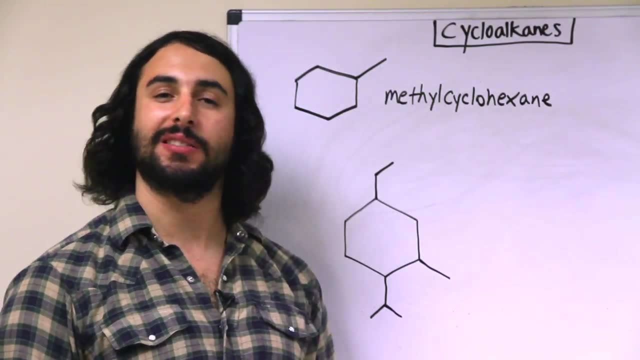 things are a little bit different with a cyclic compound compared to a linear compound because of the symmetry. now there's only one group here and it doesn't really matter where it is, because all six carbons on the cyclohexane are identical. so this is simply methyl cyclohexane. we do not have to indicate. 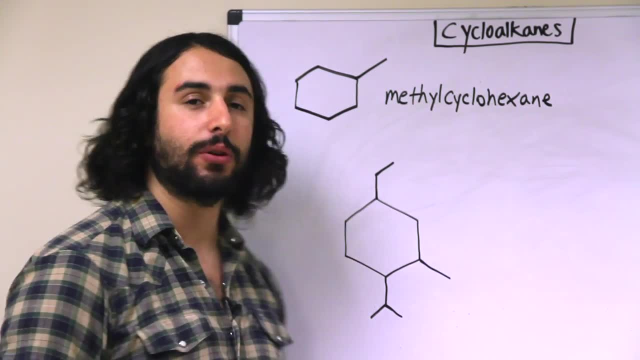 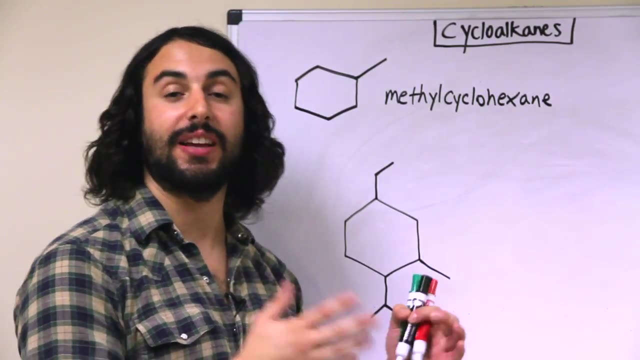 the location of the methyl group, because if it were on any other carbon, we could simply rotate it and it would be the same molecule. so this is methyl cyclohexane. that is sufficiently unambiguous. however, when there are multiple substituents, we are going to have to use a numbering system that is a. 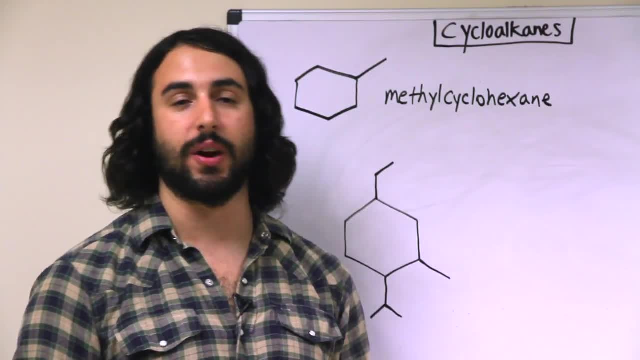 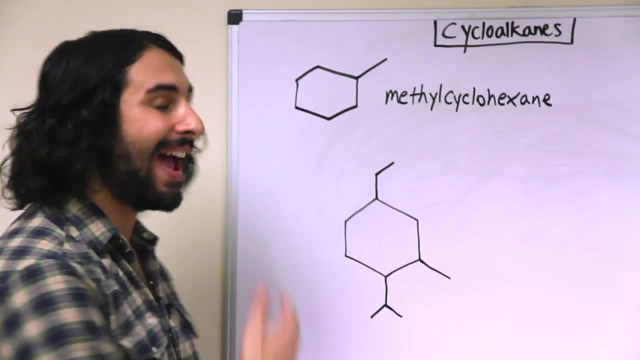 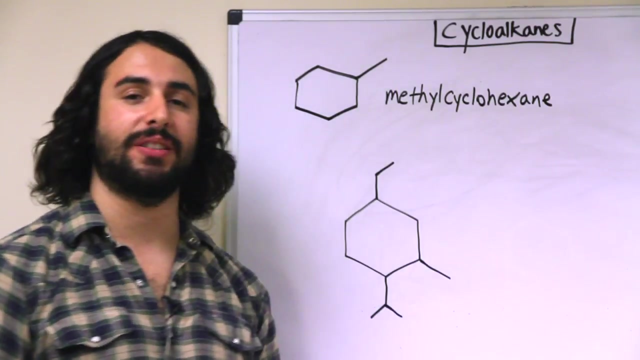 different from a linear molecule because we no longer have a situation where it is left to right or right to left. now there are actually 12 possible ways to number this ring, because we could start on any of the six carbons and then go either counterclockwise or clockwise. however, we will choose the numbering. 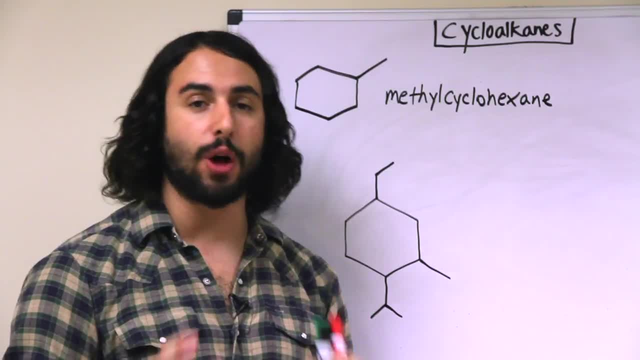 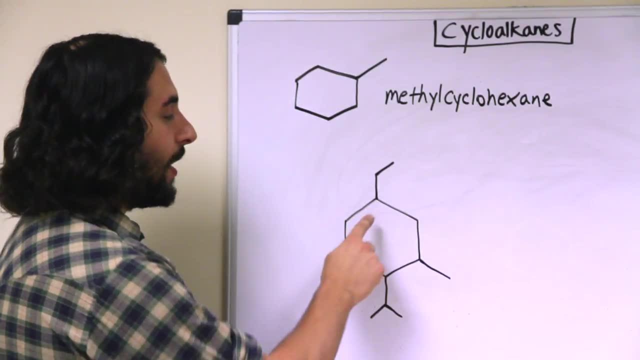 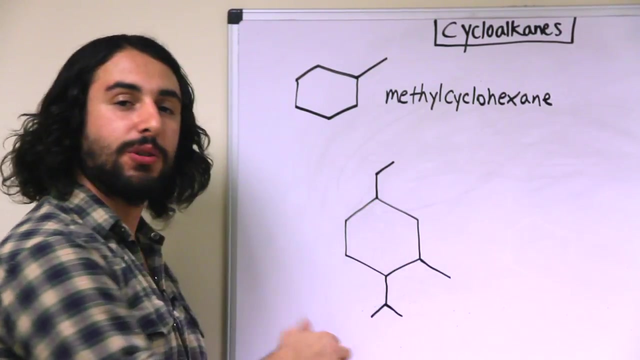 system that gives the lowest set of locants possible for the substituents that are present. so let me show you what I mean. basically, let's say arbitrarily, if we began here with carbon 1 and then went clockwise, this would be 1,, 2,, 3, and 4.. so we would have 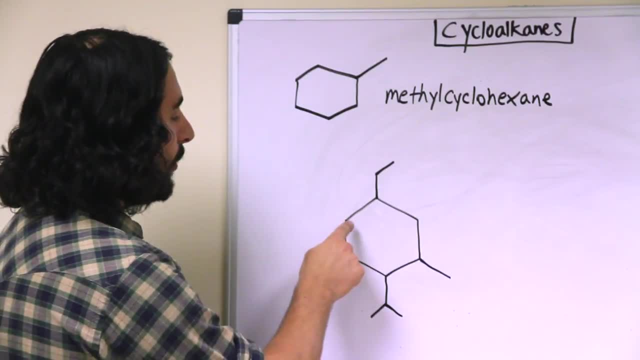 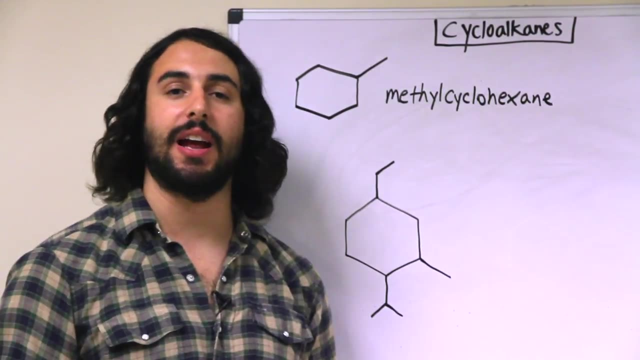 substituents on carbons 1,, 3, and 4.. let's say, we started here and went counterclockwise, we would have a substituent on 3,, 4, and then 6, right, so you can see how there are many possible sets of locants, but the one that offers. 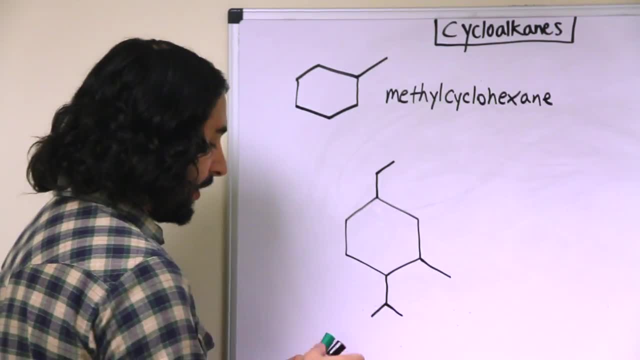 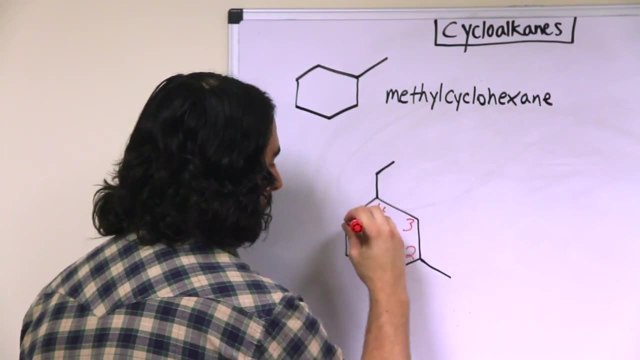 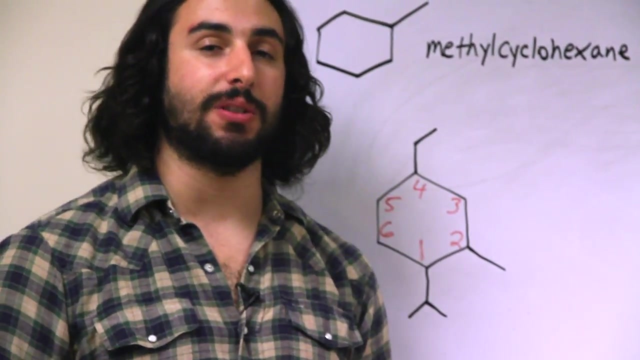 the lowest set of locants is if we begin here and go counterclockwise. now the locants are 1,, 2, and 4.. so it doesn't matter what the substituents are, at least if they are alkyl or halogen. those are equal priority. so here, 1, 2, and 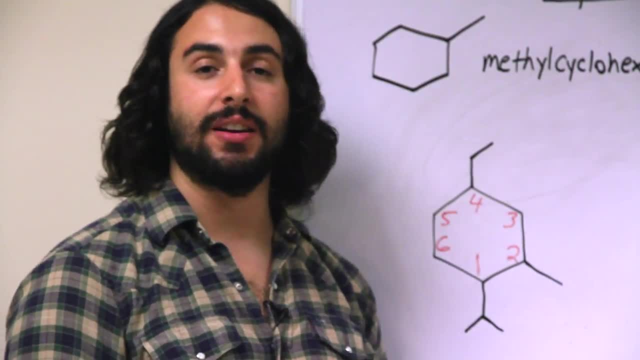 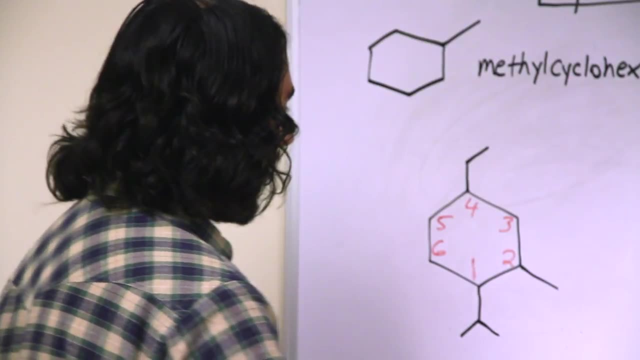 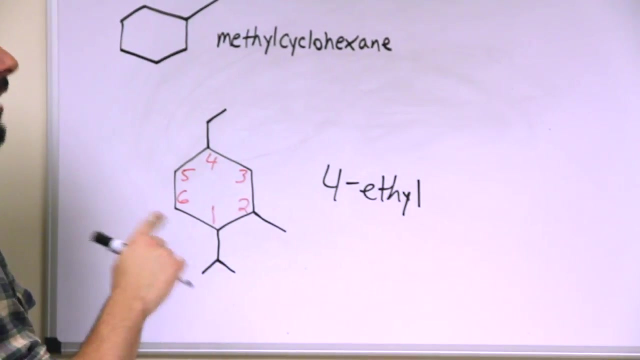 4 is the lowest set of locants possible, then by a separate algorithm, we're going to just list them alphabetically, as we always do. so 4-ethyl is going to be first and then actually isopropyl is before methyl right, because iso is the only. 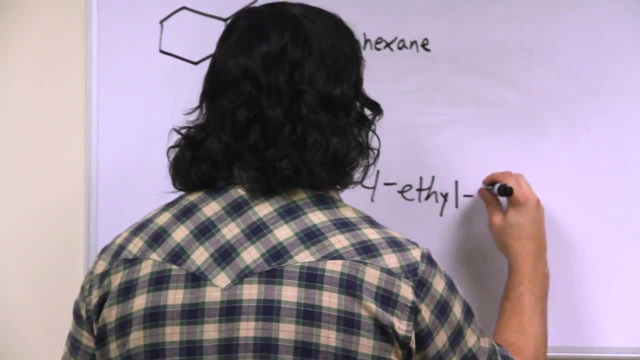 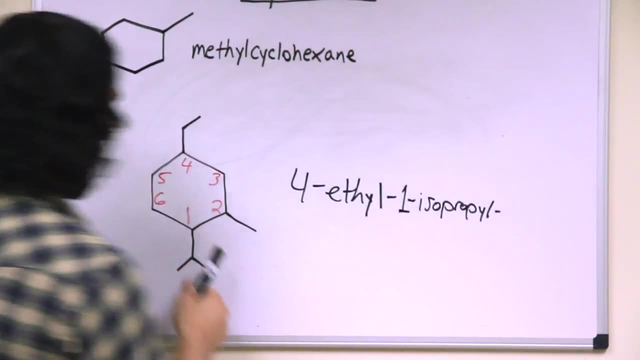 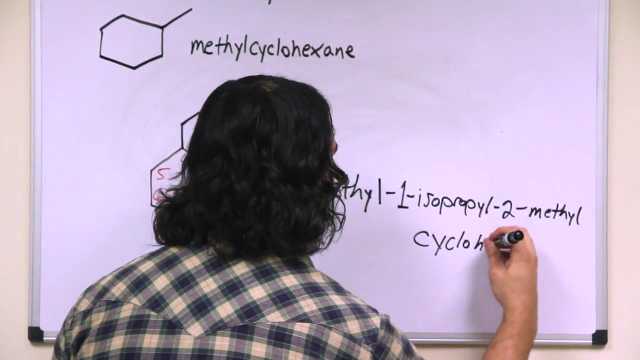 prefix that is taken into account for alphabeticity. so that's 1-isopropyl and then 2-methyl-cyclohexane. so once again we chose a set of locants that are in the lower set of locants. so we're going to. 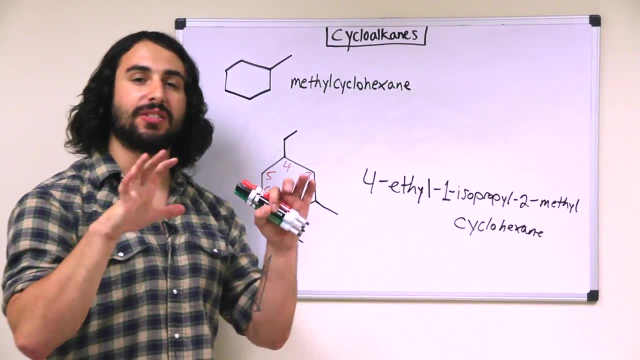 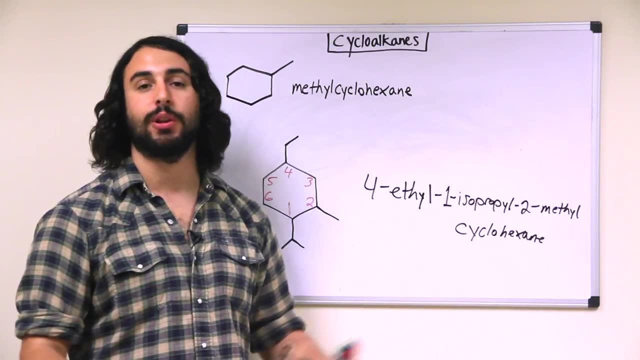 choose 1,, 2,, 4 as a numbering system, because that is the lowest possible set of locants for those substituents, and then we simply list them alphabetically, as we normally would. so we just looked at some cyclic compounds with alkyl. 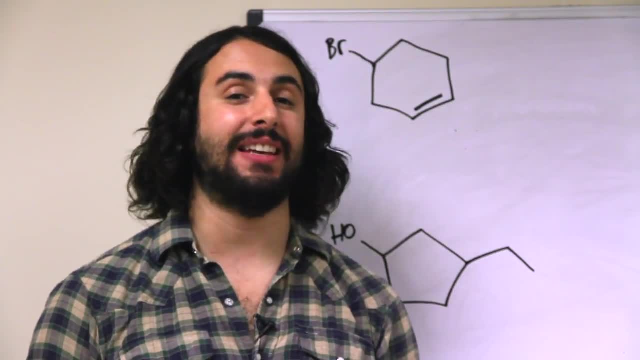 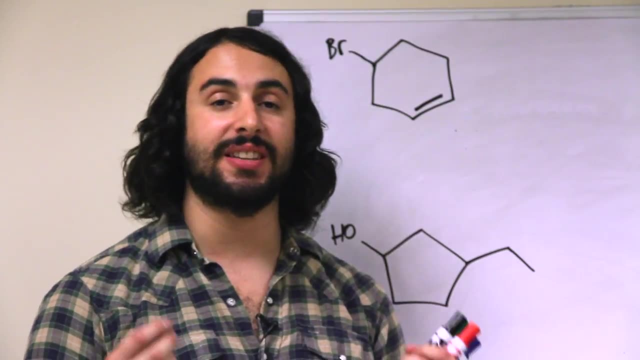 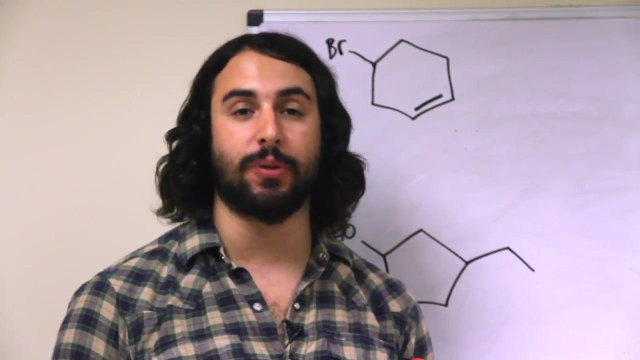 substituents. but what if we were looking at cycloalkenes or cycloalkynes, or cyclic compounds with hydroxyl groups? these are the substituents that take priority over alkyl and halogen in terms of the numbering scheme. so let's look at how we're going to apply prioritization to the cyclic. 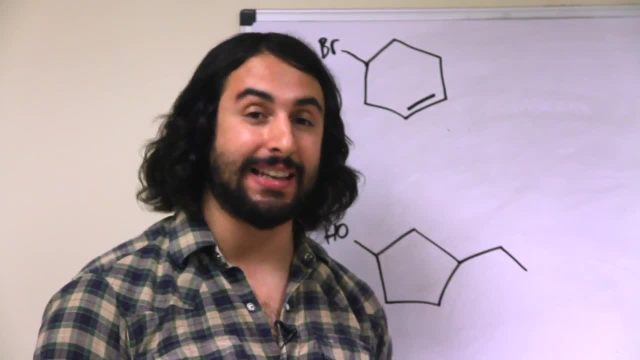 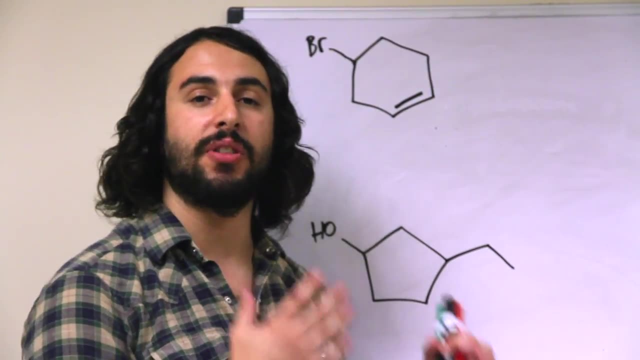 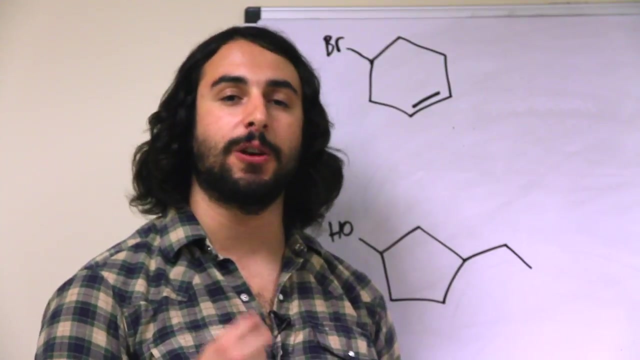 compounds. so here we have a cycloalkene, and the presence of the double bond means that we have to give prioritization to that functional group in terms of the numbering scheme. so when we have a double bond present in a cyclic compound, the two carbons that are participating in the double bond are: 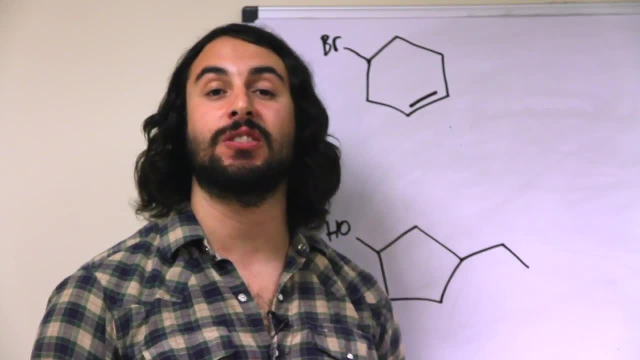 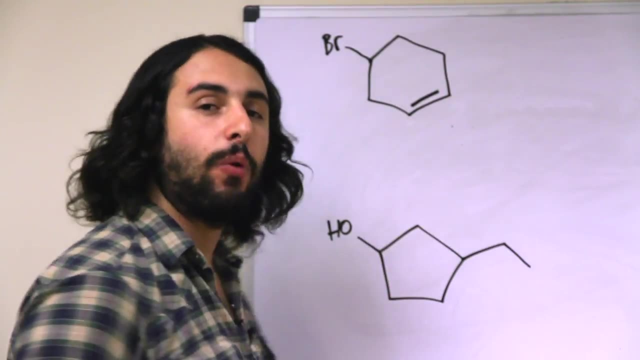 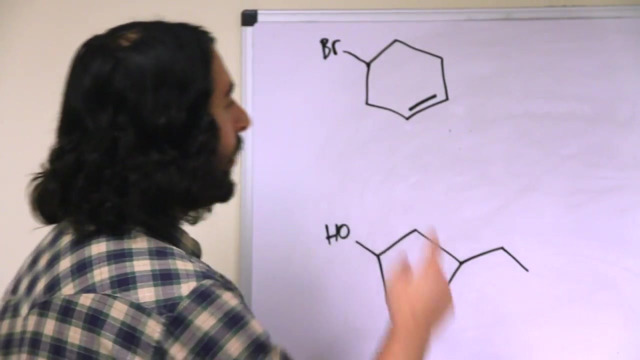 going to be carbons 1 and 2 in some order. so we have two options: either carbon 1 and carbon 2. or carbon 1 and 2.. now we will choose one of those two directions so as to give any other substituents occurring sooner. so we are going to have to number. 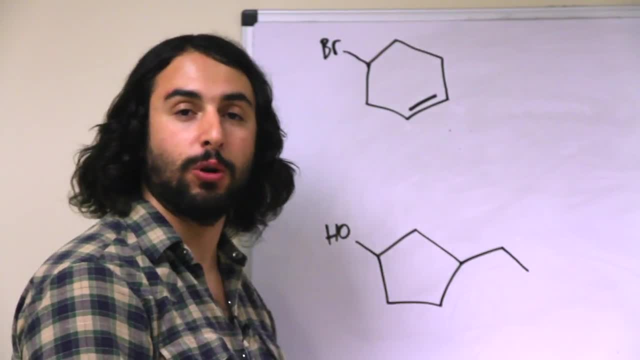 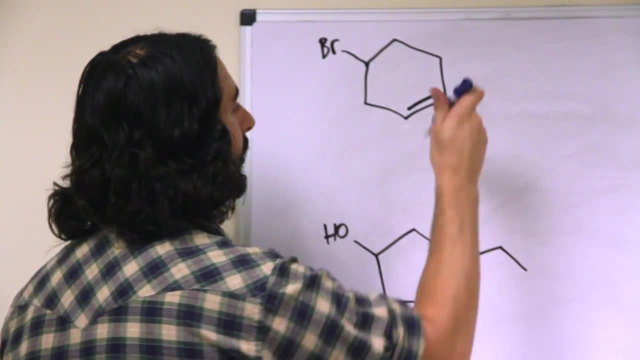 this 1,, 2,, 3, 4, because then the bromo group will occur on carbon 4, as opposed to 1,, 2,, 3,, 4, 5 occurring in carbon 5.. so that is why we will number it this way. 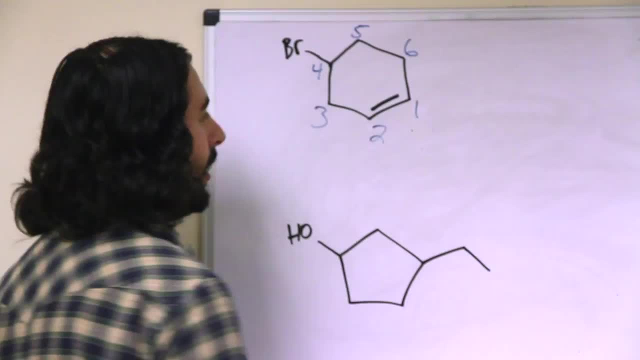 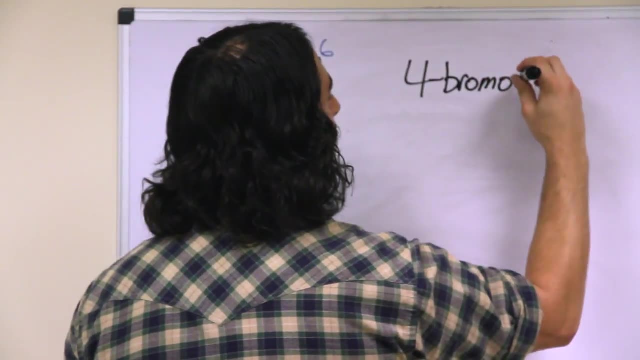 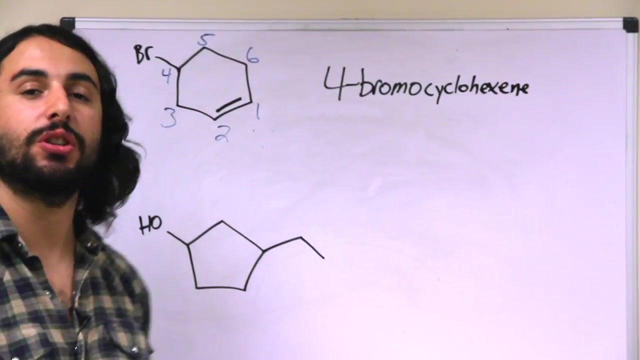 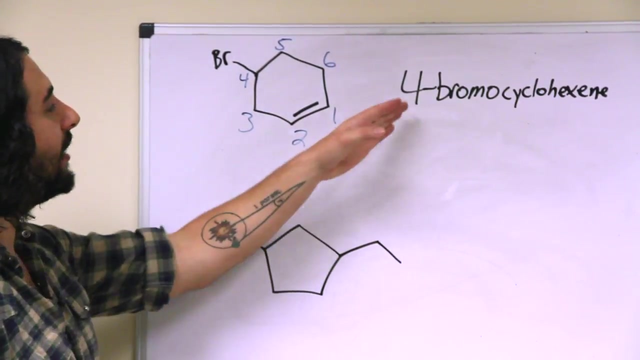 and so now we are going to list the substituent. we have 4-bromo, but then we can simply say cyclohexene, and that is sufficiently unambiguous because it is a cyclic compound. so we are talking about a cyclohexene and we are listing the location of the other. 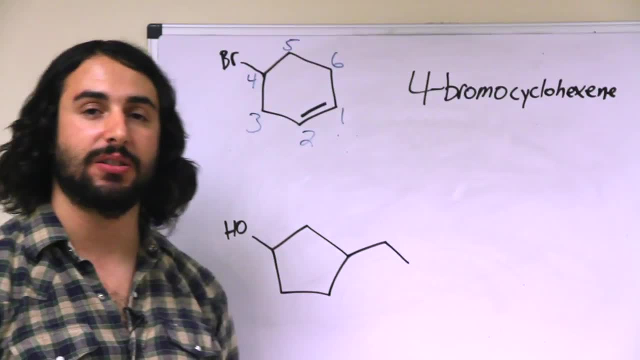 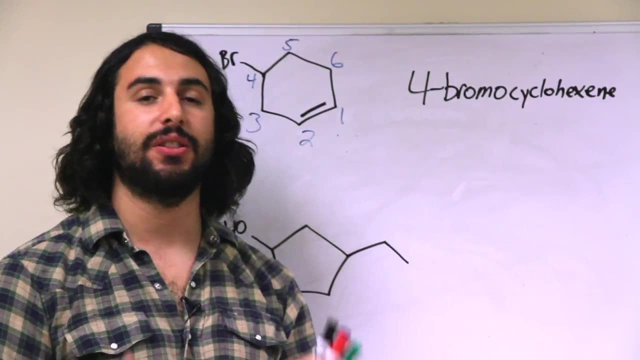 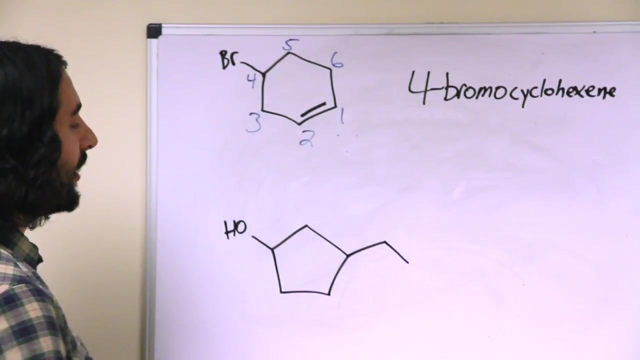 substituent in relation to the double bond. so that is sufficiently unambiguous. without saying where the double bond is, it is implied that the double bond is between carbons 1 and 2, because that is the convention we have used to number the ring. so let's look at another compound with a. 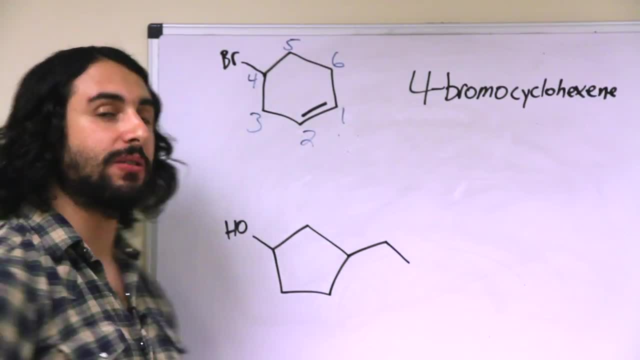 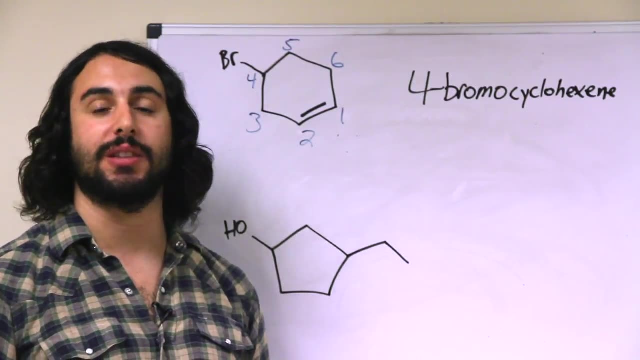 hydroxyl group. as you would expect, this hydroxyl group is going to take priority over the alkyl group in terms of numbering, so that means that the carbon that bears the hydroxyl will be carbon 1.. once again, we are going to choose the direction to number so as to giving the 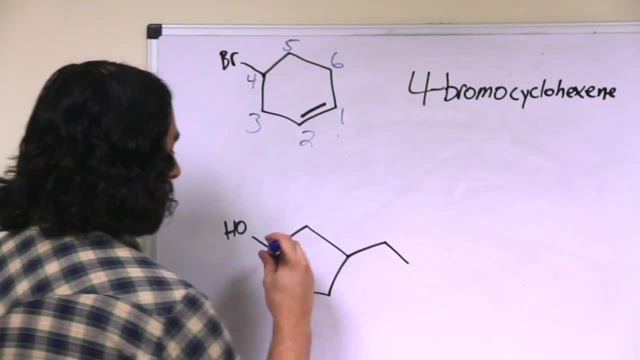 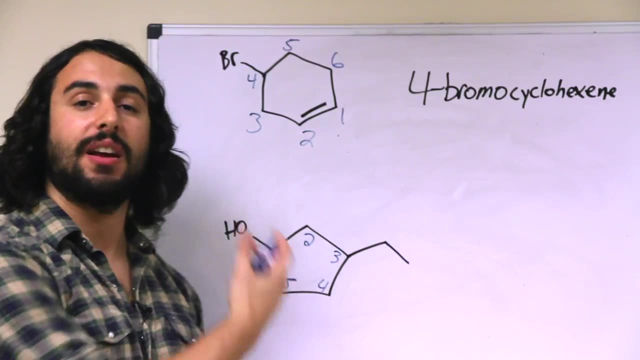 other substituent occurring sooner. in this case it is going to be clockwise because that will give the ethyl group occurring on carbon 3 instead of 4 if we went the other way. so once again we are going to say 3-ethyl. 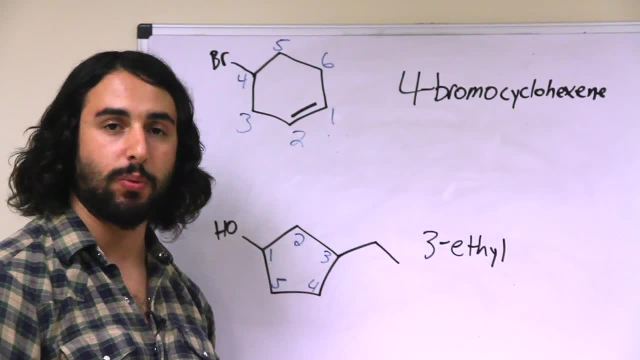 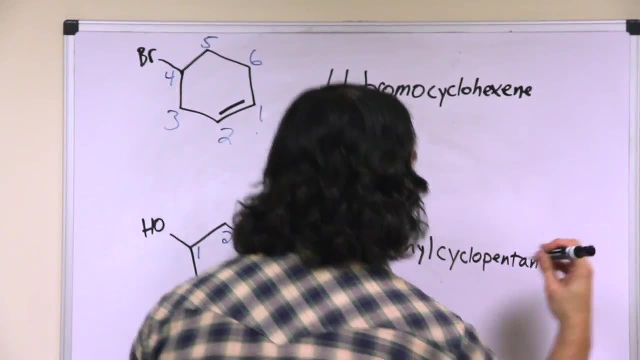 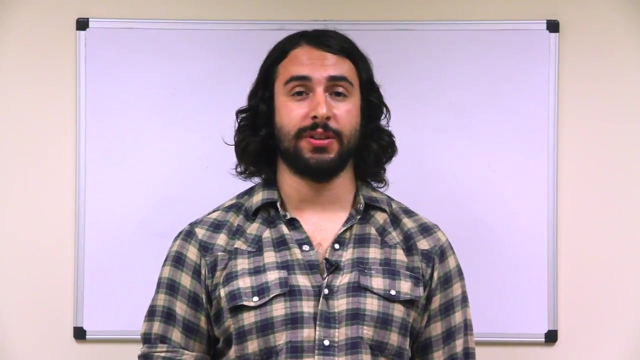 and then again it is implied that the hydroxyl occurs on carbon 1, so we can simply say cyclopentanol 3-ethyl cyclopentanol. thanks for watching, guys. subscribe to my channel for more tutorials and, as always, feel free to email me with questions. professordavexplains at gmailcom.